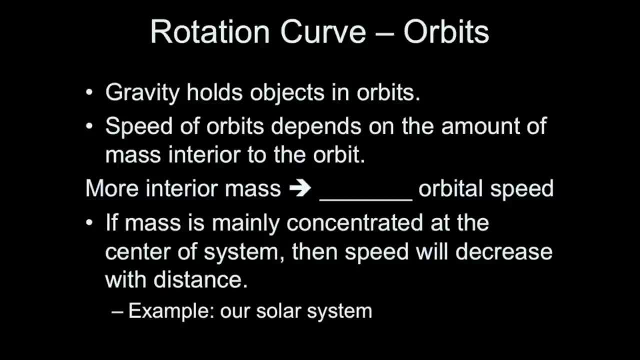 because Mongolian장을, which is a similar word for one говорит, has the same best sign of w to the R value with a greater than PO 값 which, in accordance with formulas anyone takes can bipartite. And we're also going to see in astronomy how gravity holds. 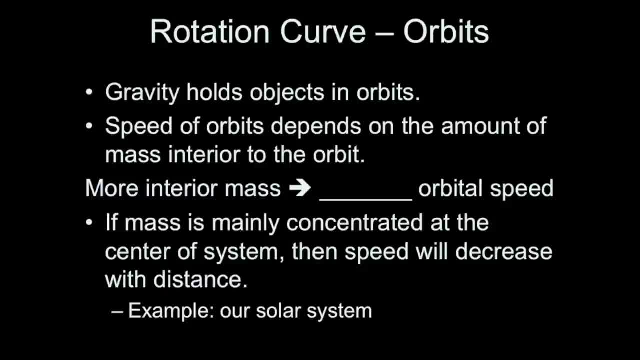 things in orbit. One of the rules that we use in astronomy is that the speed of something in orbit depends how much mass is inside the orbit. So a very simple truth about that is that in orbit there's minute wat game capacity for anything. The bigger the mass interior to the orbit, the bigger the gravitational force you'll 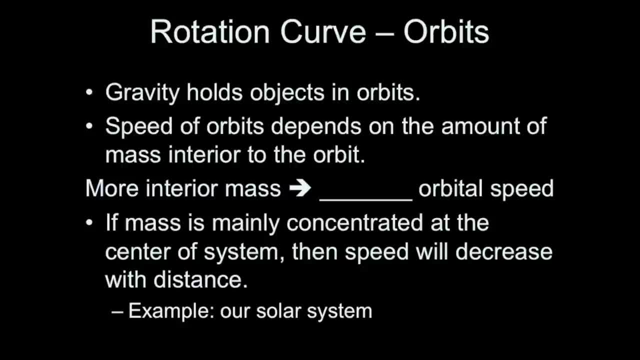 have on the orbiting object. Bigger gravitational force means bigger acceleration, bigger orbital speed. that results from this. So more interior mass means higher orbital speed. Now if the mass is mainly concentrated at the center of the system, then the speed will decrease with distance. 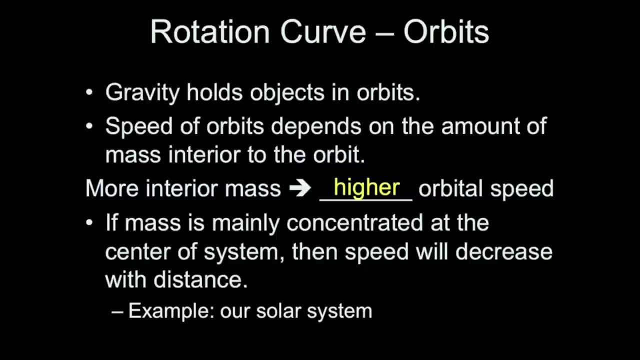 And so what that means is you'll have most of the mass concentrated in the center, For example, the sun at the center of our solar system, And as you get further away, the things that are orbiting have basically a constant amount of mass inside their orbit. 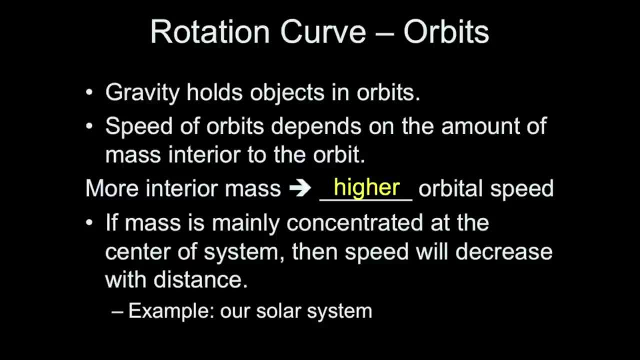 So the further away you get, the further away you're getting from the massive object and you'll have a decrease in orbital speed Because of a decrease In gravitational force. So a good example of a system like this would be our solar system. 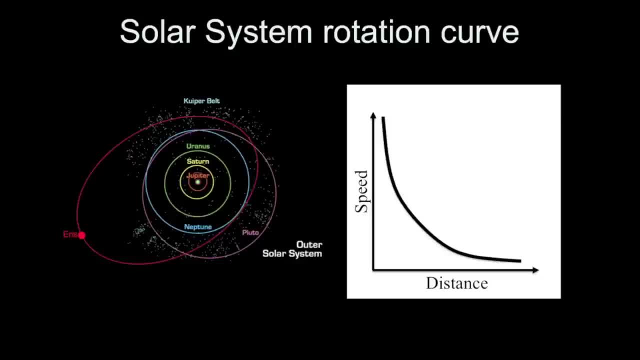 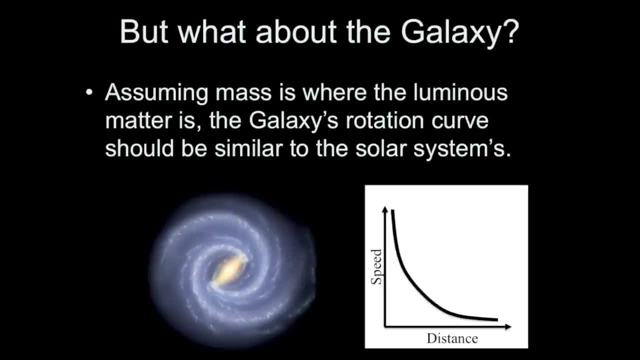 And here is the rotation curve for our solar system: As you get further out from the sun, the orbital speed goes down. But what about the galaxy? When we look at a galaxy like our own, or like other spiral galaxies, what we see is: 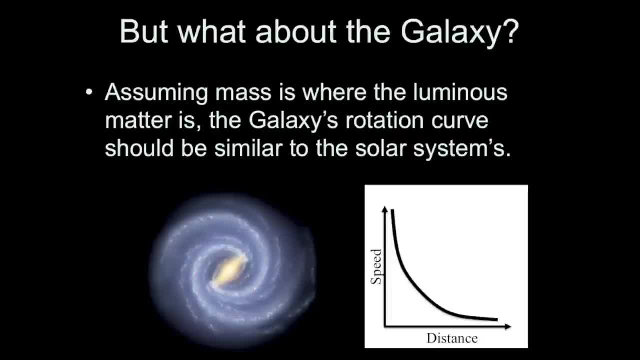 that it's. you've got more luminosity near the center of the galaxy, And so if you're just going by the luminous material, you would expect that There's more mass concentrated at the center of the galaxy and so its rotation curve should. 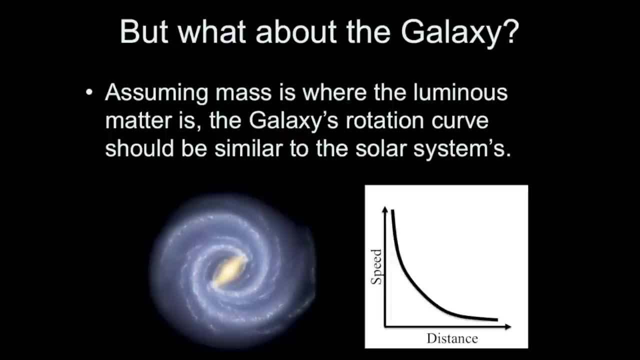 be somewhat similar to what the solar systems would be like. So you'd start with high speed near the center of the galaxy, and as you get further away from the center the orbital speed of stars and other material would go down. But that's actually not what is measured. 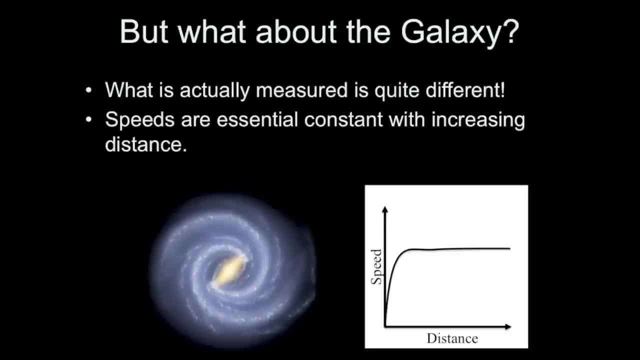 What is actually measured is very different from this, And I've drawn a Rough rotation curve for what astronomers actually measure for our Milky Way galaxy By measuring the speeds of stars and clouds of hydrogen within the galaxy using Doppler shift measurements. what we find is that the speeds of these objects as you get farther 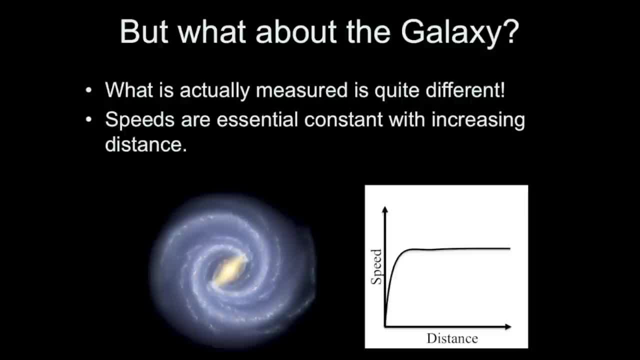 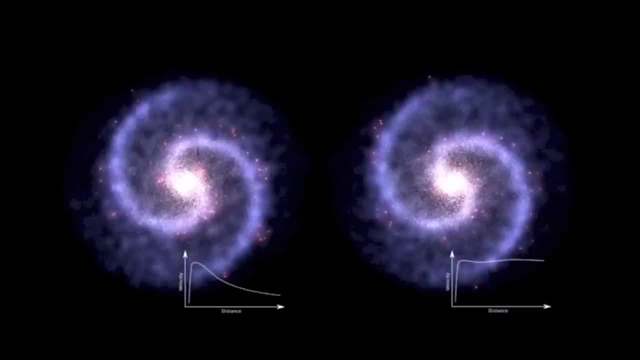 away from the center of the galaxy stay roughly constant. This is kind of strange. A galaxy in which the stars have roughly Constant speed as you get further away from the center is going to be very different in some respects than a galaxy that doesn't have constant speeds. 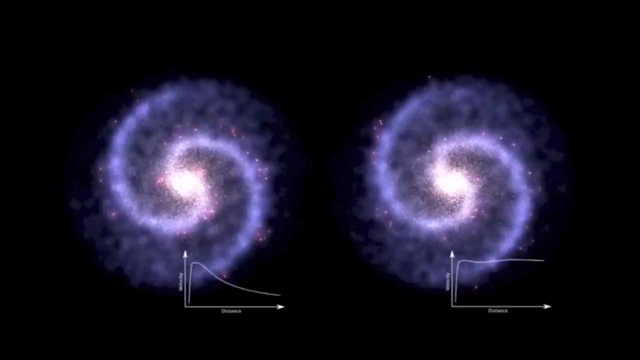 I'm going to illustrate this with an animation that shows a galaxy on the left which has its mask all concentrated at the center, and then a galaxy on the right which has its mass fairly evenly distributed as you get further away from the center. 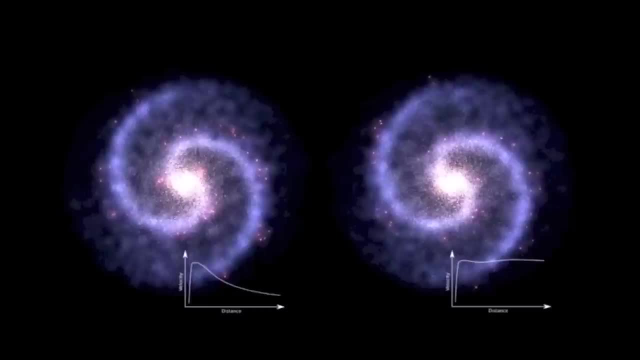 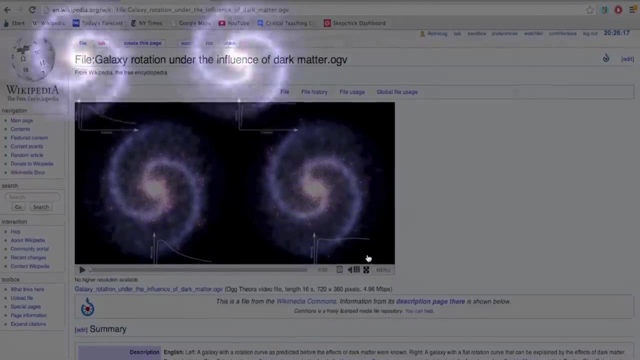 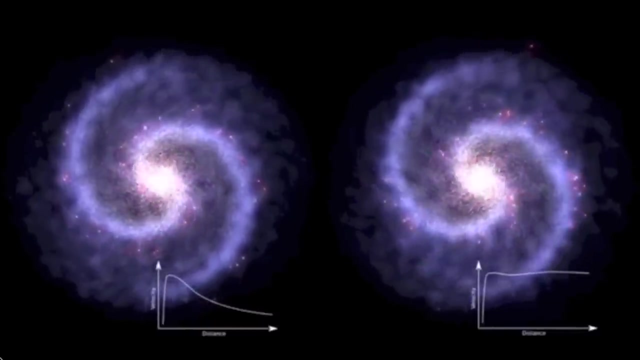 And this allows for a constant orbital speed the further away you get from the center of the galaxy. So what we see on the left is a galaxy that has orbital speeds slower as you get further from the center, And on the right Is a galaxy. 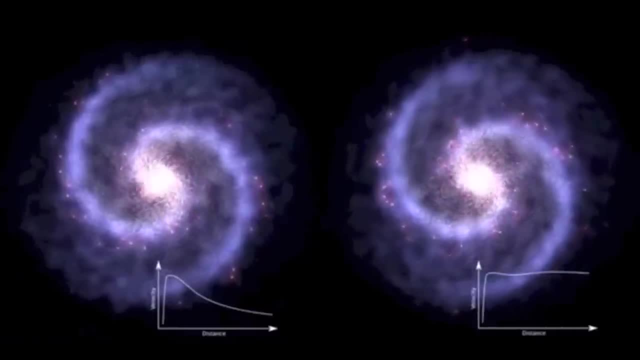 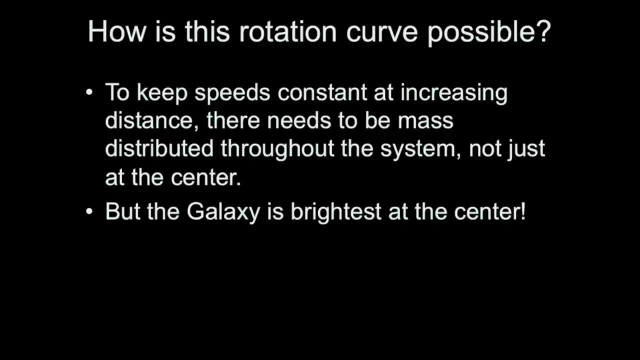 That stays constant further from the center. So how is a rotation curve like that possible? In order to keep the speeds constant at an increasing distance, there needs to be mass distributed throughout the entire orbital system, not just at the center. But, you might ask. the galaxy is brightest at the center. so what is this other mass? 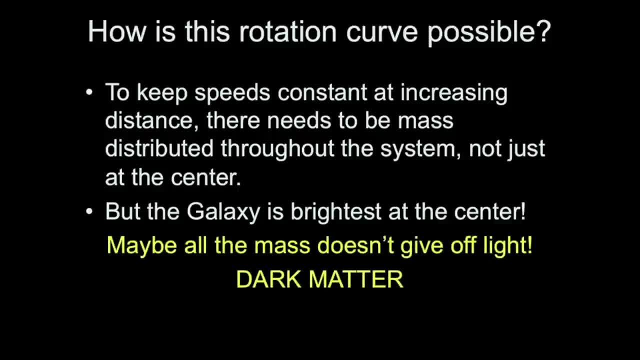 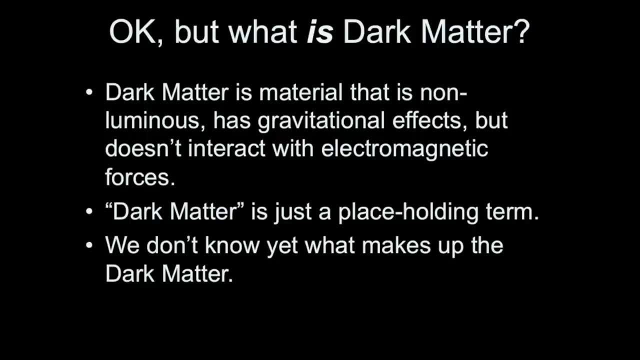 Well, that's a problem, Unless We consider that perhaps all the mass of the galaxy doesn't give off light, And so that leads us to the idea of dark matter, That there's additional mass within our galaxy that isn't luminous. But what is the dark matter? 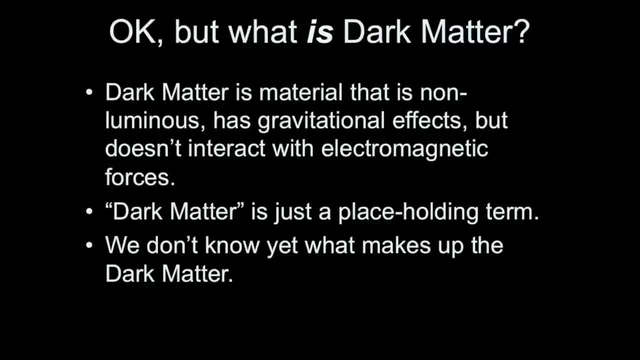 All we mean by that is that dark matter is material that is not luminous, That is, it's not giving off light. It has gravitational effects but doesn't interact with extra light. Dark matter is material that doesn't give off light. 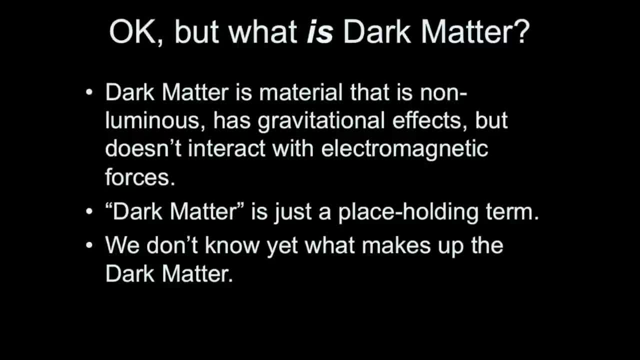 It's not luminous. It does have gravitational effects on the things around it, But it doesn't interact with other things using the electromagnetic force. The term dark matter is just a place holding term that we're using to describe this material until we figure out what the particles are or what the material is. 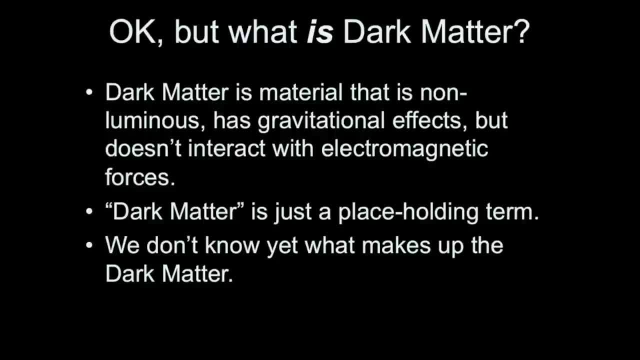 We don't really know yet what makes up all of the dark matter. There's a lot of different ideas that astronomers and particle physicists have. But we don't know yet what makes up all of the dark matter. There's a lot of different ideas that astronomers and particle physicists have. 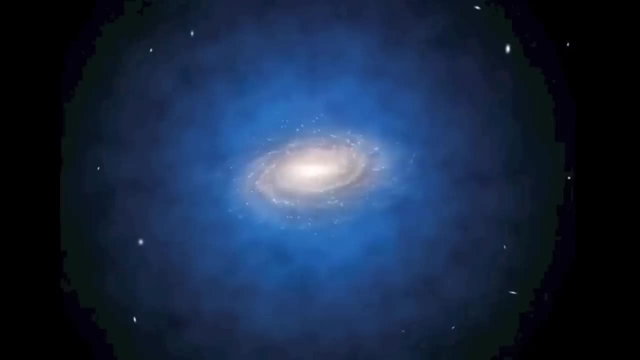 But we don't really know yet what makes up all of the dark matter. There's a lot of different ideas that astronomers and particle physicists have. This image that I'm showing you is a depiction of what the Milky Way might look like from the outside, including the luminous matter. 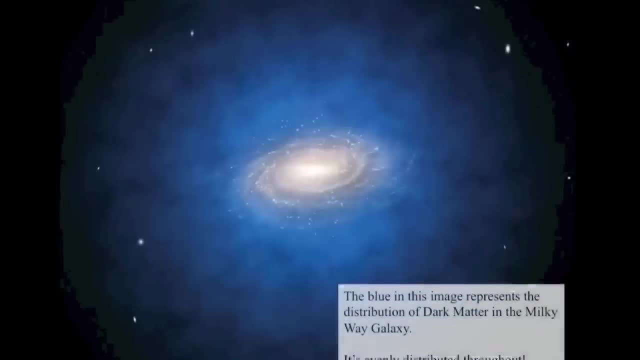 But then the blue color that you see shows the distribution of where the dark matter would be in the galaxy and throughout the halo of the Milky Way galaxy. It's evenly distributed throughout. It's evenly distributed throughout. further away from the center, you have an increase in mass interior to the orbits of 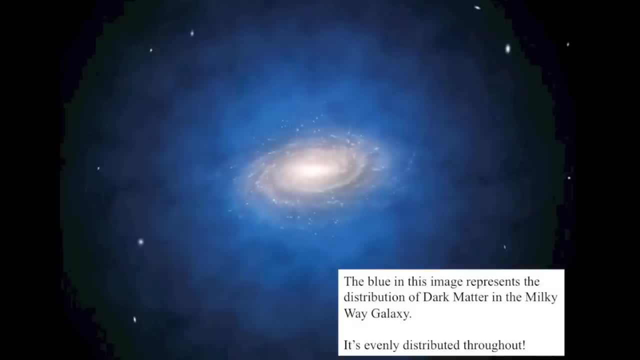 those stars. This means more gravitational force as you get further away, and that means the stars that are further out are able to maintain high orbital velocities. We don't notice this just for the Milky Way galaxy. We see this in other galaxies as well. 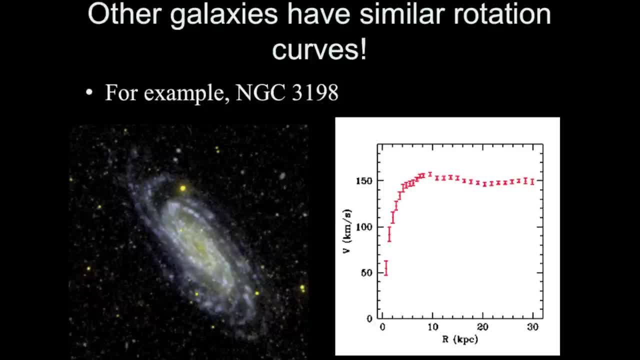 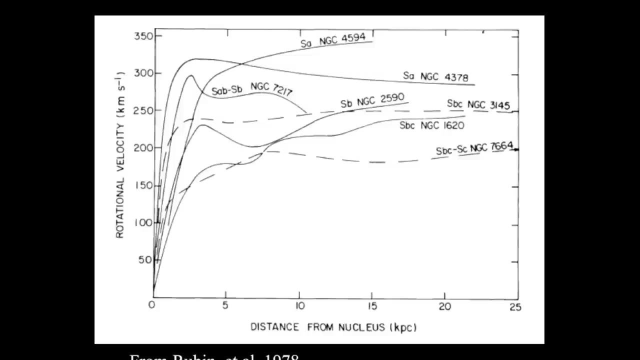 So, for example, on the left is an image of NGC 3198, and on the right is its measured rotation curve. Again, this is very similar to the Milky Way's rotation curve, where you have a roughly constant orbital speed the further away you get from the center. 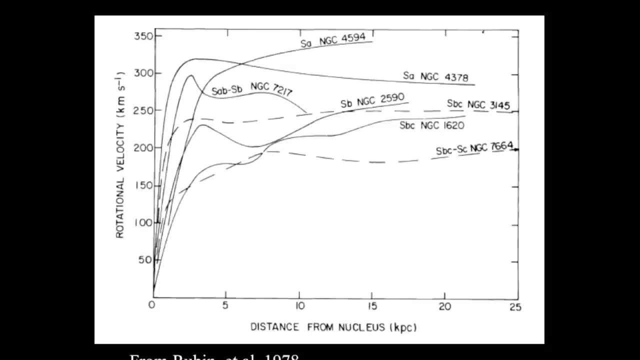 Other galaxies as well show this same pattern of rotation curves. This is an image that comes from a peer-reviewed journal publication from Vera Rubin and her collaborators that was published in the late 1970s. Vera Rubin- Vera Rubin did a lot of the work in the 1960s and 1970s measuring the rotation curves of